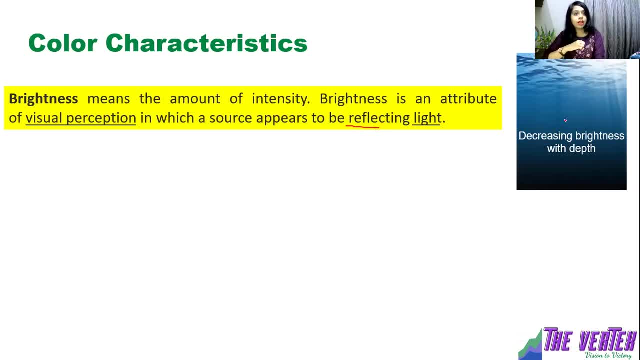 light is more and hence brightness will be more. and when we go deeper into the water, the reflection of light will be less, and that's why the there you will say you, you can see less brightness. that means this: intensity of color, or you can say amount of intensity or brightness, depends on how much light is getting. 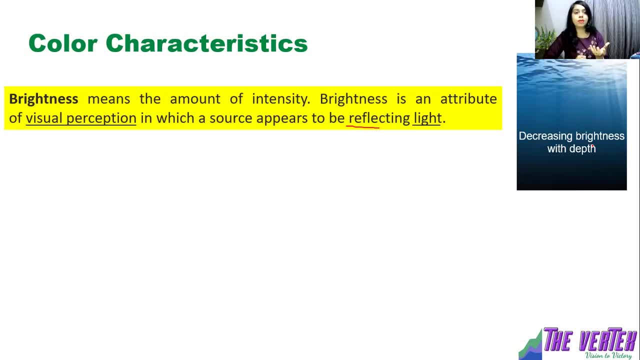 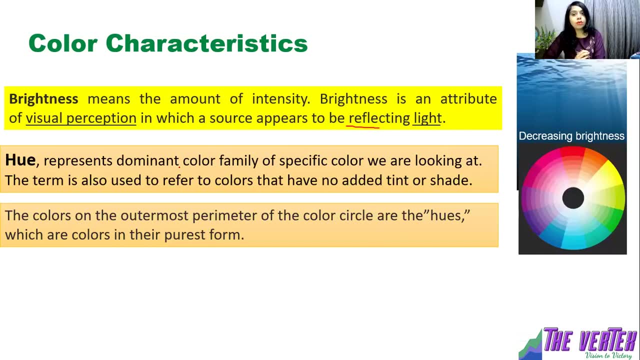 reflected. more is the reflection, more is the brightness. now, next characteristic is you. what is you? you represents dominant color family of a specific color we are looking at. so what is you? you is the dominant color of a particular color family. you can see here the color on the outermost perimeter of the color circle. 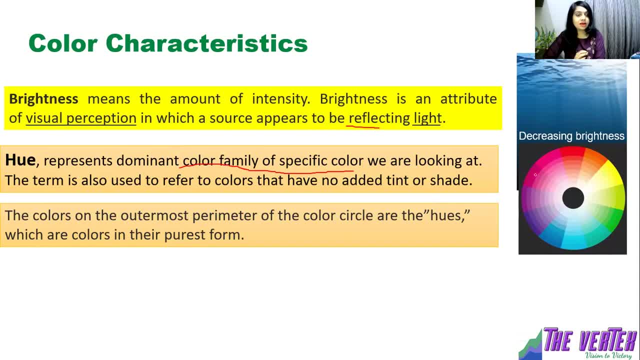 are used. you can see here, this is the. this is a color circle. you can see your outermost perimeter. so if you see, concentrate on this. if you say this is a red color family, where in red is dominant on the outer circle, or you can see here, this is a family. 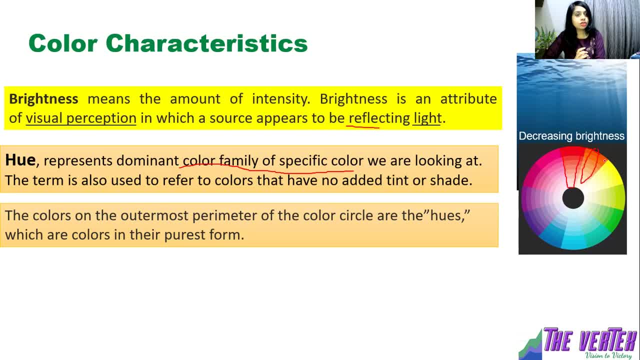 of orange color, so outermost color shows the dominance or yellow color or green color family, so outermost you can see a dominance of particular color or dominance of that particular color family and that is known as you so colors on the outermost perimeter, that means all. 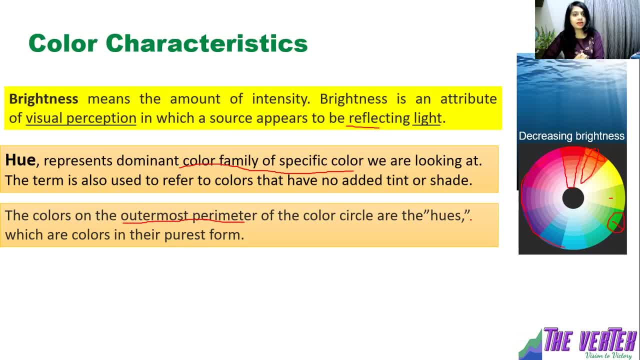 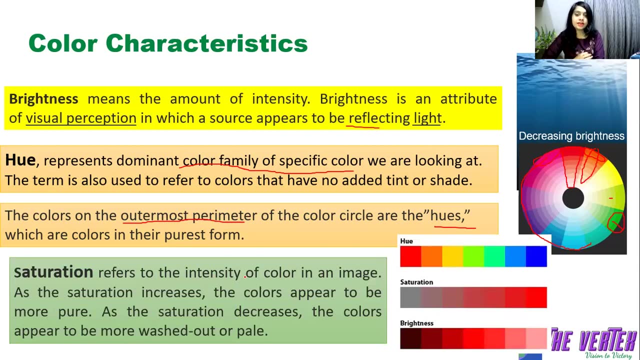 the colors on the outermost perimeter of this color circle are used, which are colors in the purest form. so these are purest form of colors. now, next characteristic is saturation. what is saturation? saturation refers to intensity of color in image. means how much is the intensity, or you can say how much is the level of color. 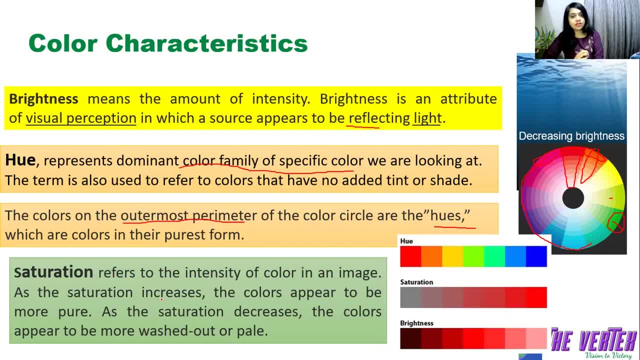 in that particular image as saturation increases. you can see here an example. as saturation increases, the color appears to be more pure form, so more is the saturation you will get that color in the more pure form. this is a pure form of red color. as the saturation decreases. 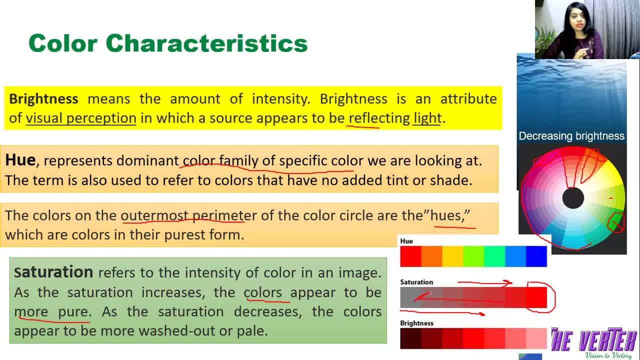 you can see your saturation is decreasing in this direction, and here you will get pale colors or washed out color of the same family. so these are the three characteristics of color, that is, brightness, hue and saturation. so now let's see what is saturation. saturation is the color of the image. 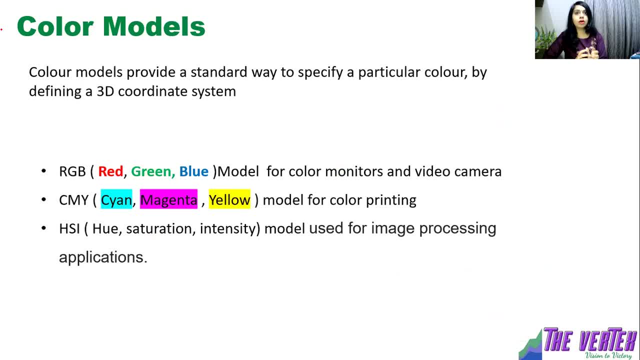 now there are three or there are different color models here. in this video we are concentrating on three main or important color models. the first is rgb color model. rgb stands for red, green and blue and these are used in monitors of video cameras, color monitors and video cameras. 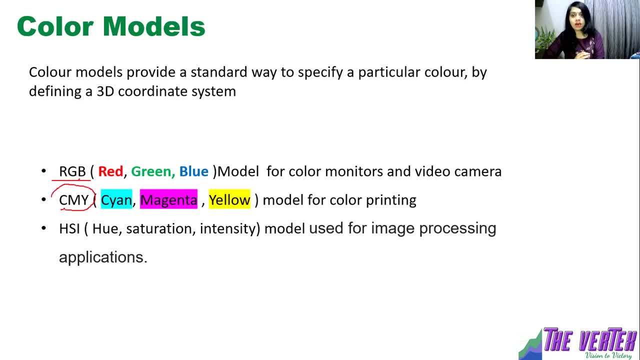 then second color model is cmy stands for cyan, then magenta and yellow. this color model is used for color painting. and next is hsi, that is hue, saturation and intensity color model. this color model is used in various applications of image processing. so color models, what color models does color models provides a standard way to specify. 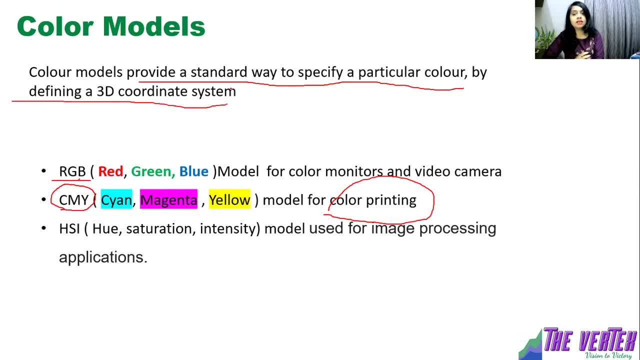 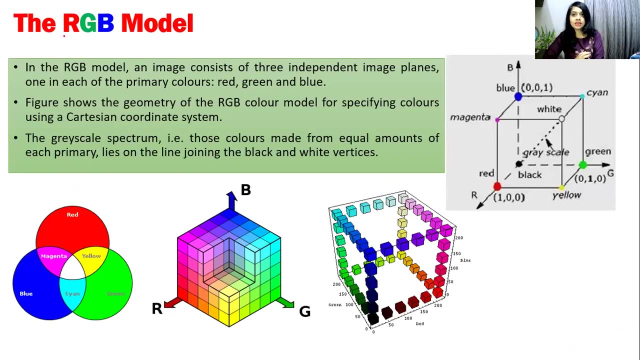 a particular color by defining a 3d coordinate system. so these colors are represented in the form of 3d coordinate system. let's see one by one. so let's start with the rgb model. so what is the rgb model? rgb as name suggests it stands. 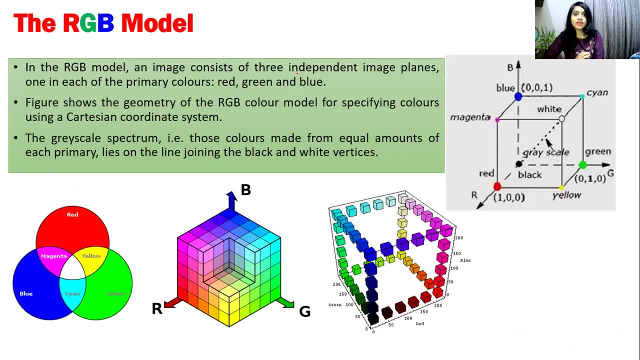 for red, green and blue model. an image consists of three independent image planes. so there are three independent image planes you can concentrate here: this is red, here it is green and here it is blue. if you see in the in this image, this is red, this is green and this is blue. 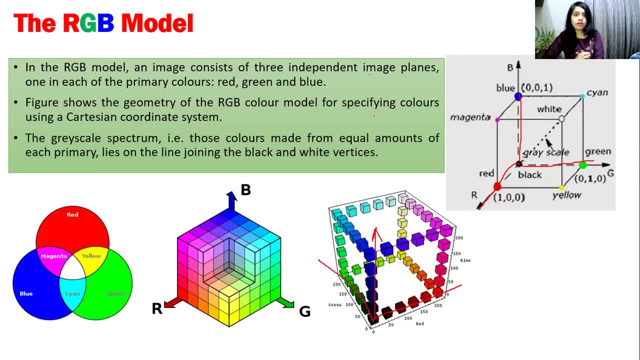 what happens. figure shows the geometry of rgb color model for specifying colors using cartesian coordinate system. now you can see, here it is. this red plane is represented by one zero zero. so what this one represents? one represents the presence of red color, and this represents absence of green color, and zero represents absence of green color. 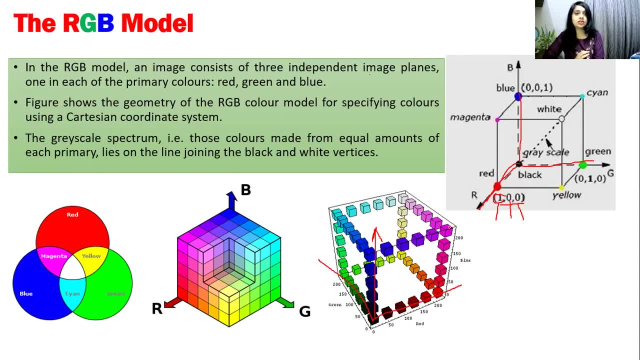 so if you see this blue plane here, it is zero, zero. this first zero indicates absence of red color, this indicates absence of green color and this represents presence of blue color in this direction. so blue is present in this direction. you can see here. blue is present in this direction. similarly, it goes for green. if you see this green plane here. 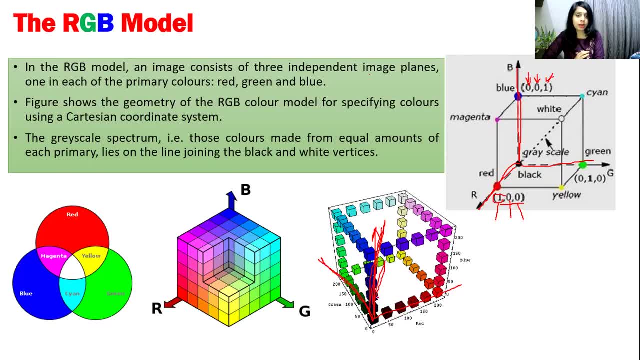 it indicates presence of green color, absence of blue color and absence of red color, and that's why r is zero, g is one and blue is zero. so this is how we can represent colors into this cartesian coordinate system. now you can concentrate here. let me take a color change. yeah, now, if you see here, you. 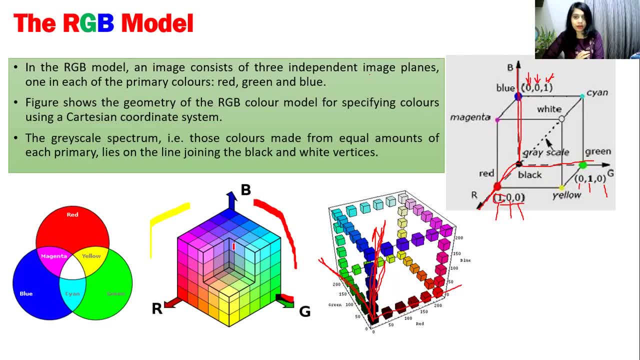 can see this: this is a green plane, this is red plane and this is blue plane. when we mix blue and green, you get. so when we mix red, sorry, when we mix blue and green, what do we get? we get cyan. so here you can see this cyan color. similarly, if you see in this direction, there is in this: 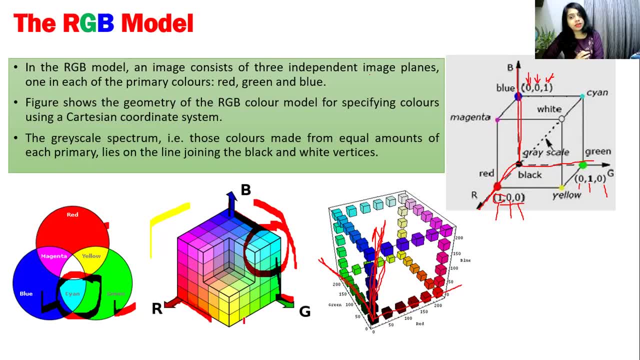 direction the red color is getting mixed with green color. so when green color gets mixed with red color we get yellow, and hence in this coordinate system you can observe, here there is yellow color, but in this direction there is absence. when this is a blue, particularly blue plane, on the blue plane. 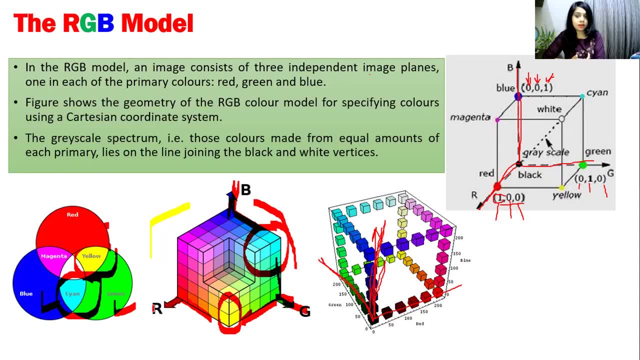 uh, the red and green are absent. in green plane, the red and blue are absent on. in the red plane, the blue and green are absent. the grayscale spectrum, those color made from equal amounts of each primary, lies on the line joining the black and white vertices. so here you can see. 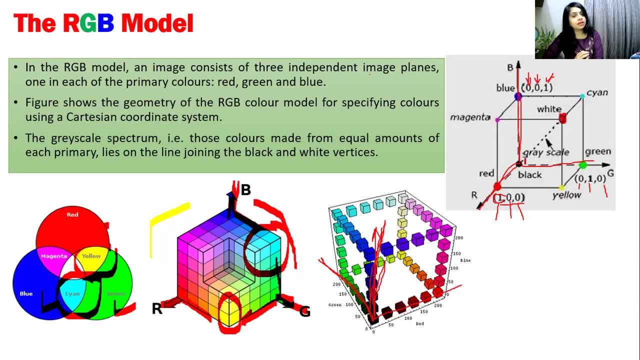 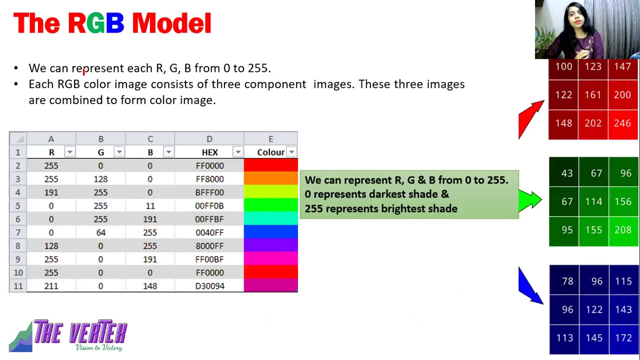 there is a white vertex and vertex and here there is a black vertex and this line indicates gray color. where do we use the rgb model? the rgb model is used for color monitors and video cameras. now, the rgb model, we represent each rgb from 0 to 25. that means each, uh, each shade, i can say each shade of. 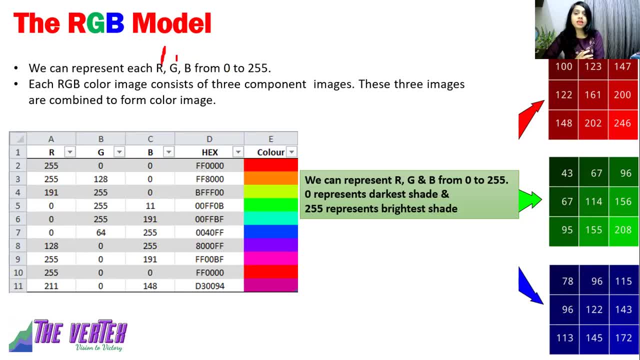 r can be represented from 0 to 255, each shade of green can be represented from 0 to 255 and blue can be again represented by 0 to 255. if you observe here, if you observe here, you can see that darkest means lesser value. smaller is the value. 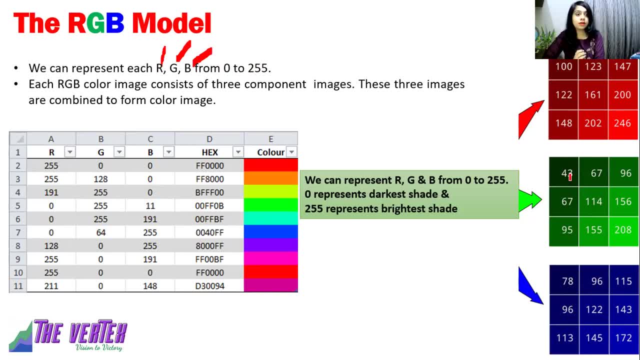 it goes towards black or darkest shade of that particular color, and when it goes towards 255, it is the more brightest of your form of that particular color. similarly, you can see here 78, which is more close to 0, and hence it is the darkest shade of. 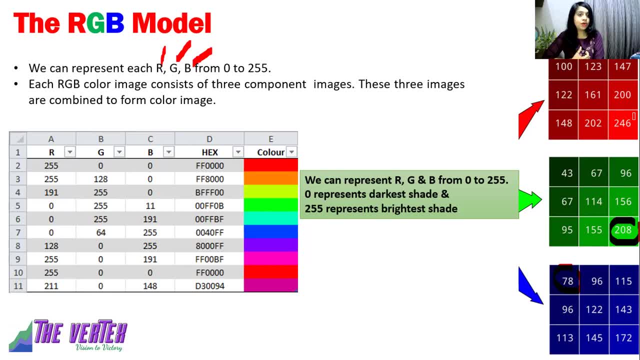 blue. in fact, if you see here this 246, 246 is uh like highest value, so it is close to uh or it is brightest shade of red. so each RGB color image means every color image consists of three component images. that means every color image is addition of these. 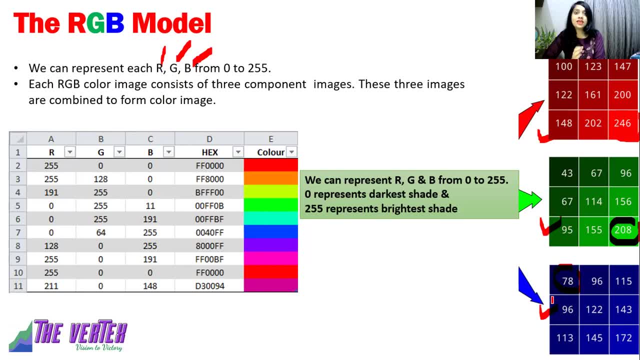 three images: one, two and three. that means each color image is addition of red plane, green plane and blue, and when we are these three we get a color image. now the intensity of every color is represented by a number from 0 to 255, and hence each can be represented by 8 bits. so if I want to represent 122, I 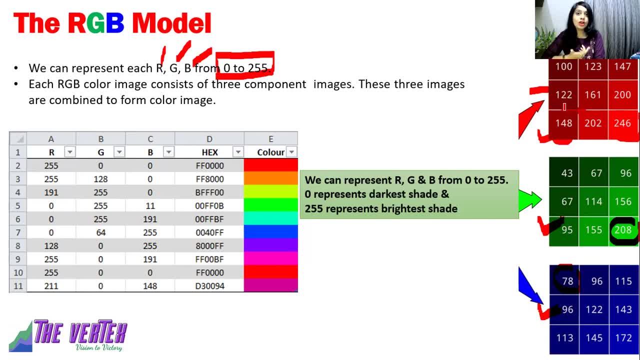 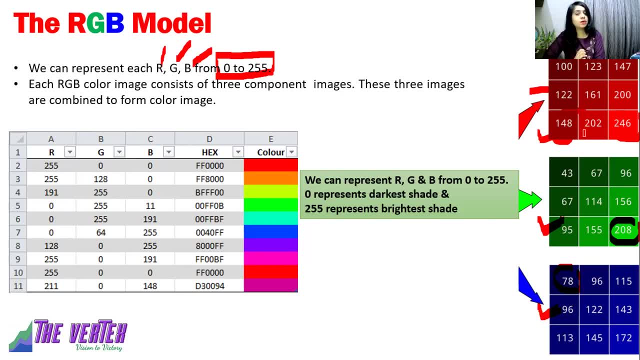 1, 1, 1 and all other shades of this particular colors can be represented by that bit patterns, which are that are a sequence of zeros and ones. now here you can see the example here: red is 255, the green is absent and blue is also absent, and hence 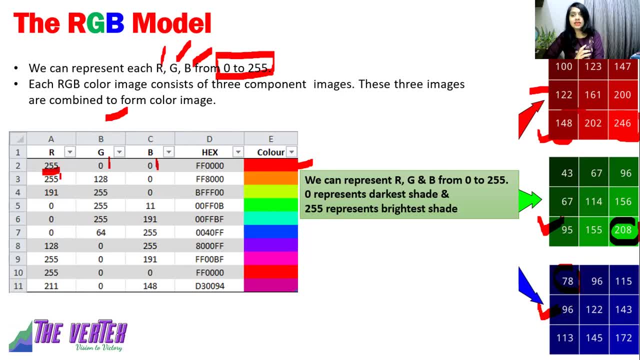 it is in the form of pure red color. here you can see that red is 255, the green intensity is 128 and blue is absent, and hence it is like this. somehow you can see that red is like orange color. here it is 191. green is 255. 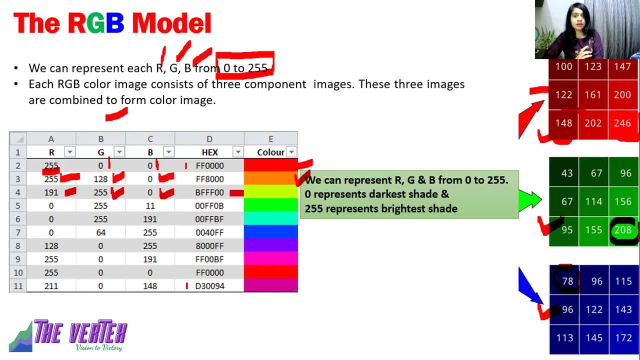 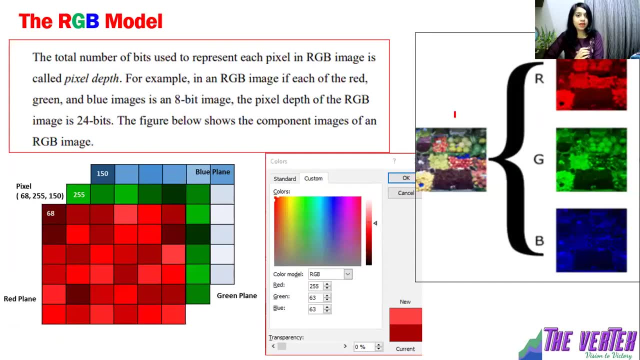 and blue is absent, so it is yellow color and so on and, as I said, it is also represented by hexadecimal numbers. now, as I said, every image, every color image, is addition of three components of RGT. so you can see here, this is a red component, this is green component and this is blue component. when we are going to do some, 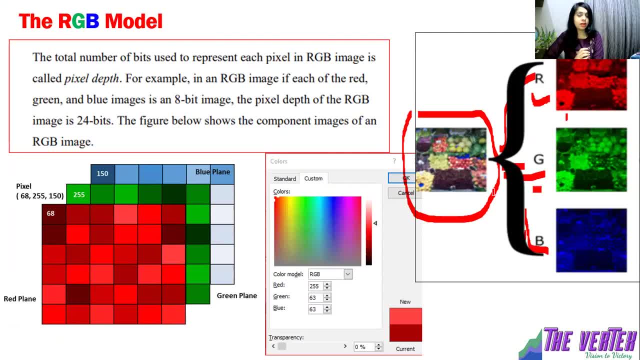 And when we add these three images, we get this particular color image. You can see- I have shown here the example. What is written? The total number of bits used to represent each color pixel in RGB image is called as pixel depth. What is the meaning of this? 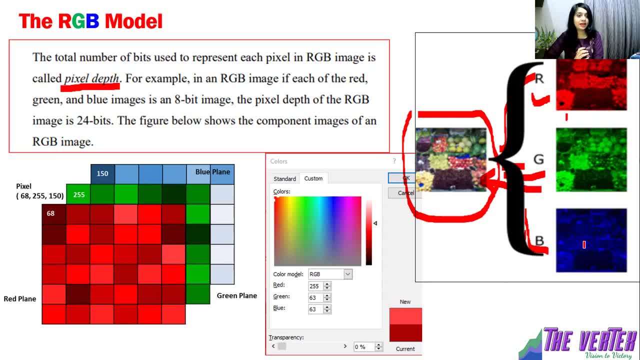 As I said, each color image consists of addition of red, green and blue plane. So here I have shown- this is blue plane example- green plane and red plane. There are different color shades varying from 0 to 255.. Here, if you take this particular pixel, this particular pixel and this particular pixel, 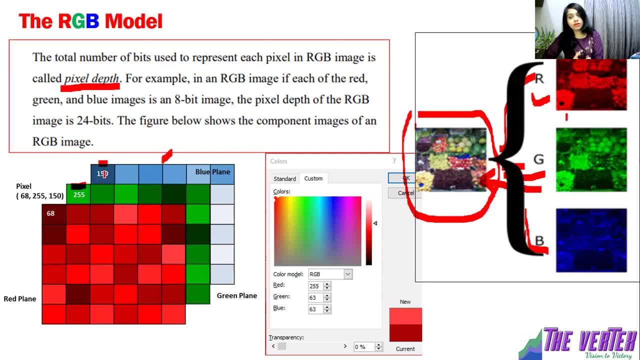 And if you see this corner pixel. corner pixel is addition of or it is represented as pixel 68R. G is 255 and blue value of blue pixel is 150.. That means each pixel of color Image have has a depth of 24 bits, because to represent 68, I need 8 bits to represent 255 of green. 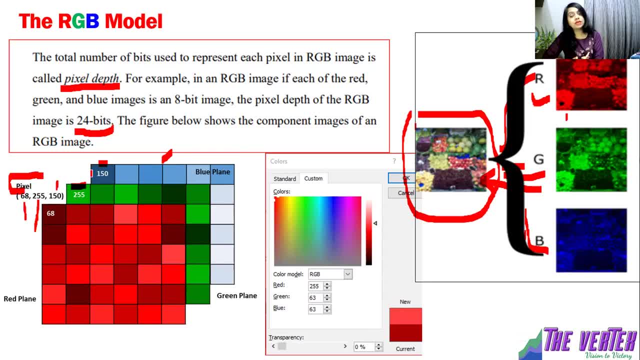 We need 8 bits, and to represent 150 of blue, We need 8 bits, and in color image it is 68 comma 255, because it is addition of all these three, and hence, to represent a color image pixel, We Need 24 bits, and hence it is said that the depth of RGB image is 24 bits, and so on. 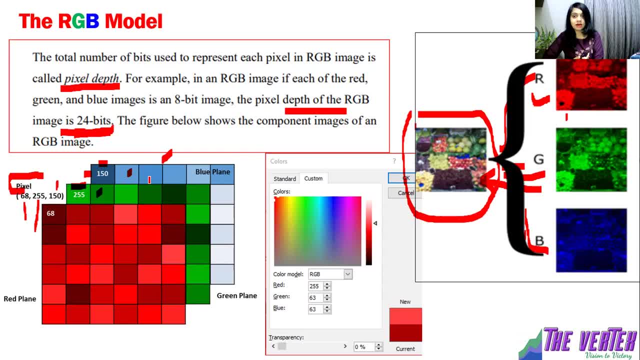 The second pixel will be addition of this, this and this. The third will be addition of this, this and this, and then so on. So these are different planes of images. If you open a Microsoft PowerPoint and if you add this- any of the color that you want to use, either for the text or as a background, you will see it opens this text. 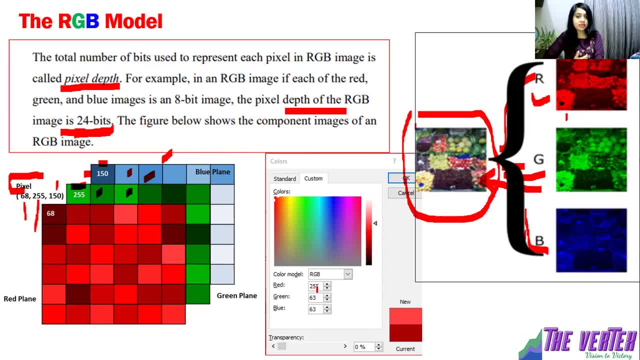 The third one is a text box And when you add does this arrow, it will change the value of RGB. So what is this value of RGB? It is nothing but these values of RGB. Whenever you want to select a particular shade of, say, red or green or blue, it will change the intensity, or you can see the level of red, green and blue. 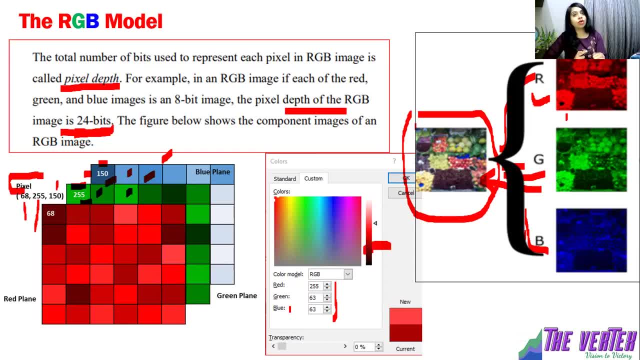 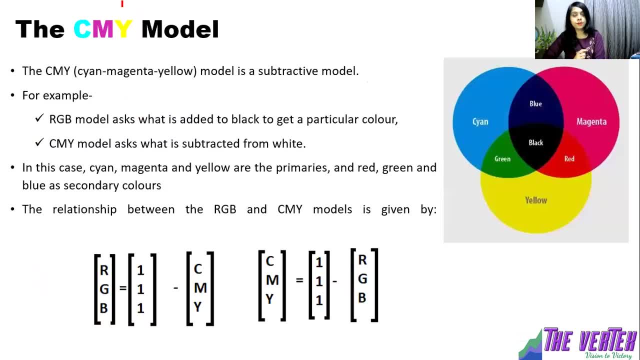 So remember, every color image is addition of three image components, That is, a Red component, blue component and green component. Now, next model is CMY model, That is cyan, magenta and yellow model. This is subtractive model. What is meaning of subtractive model? 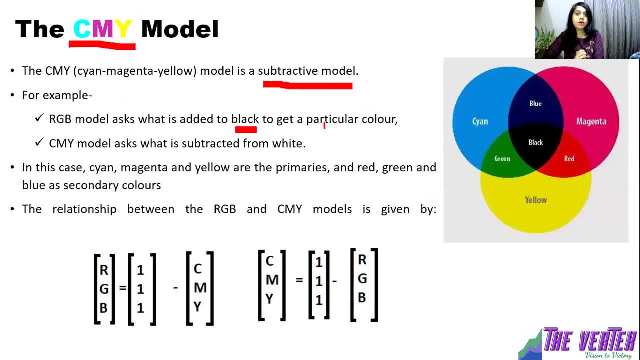 RGB model asks what is added to black to get particular color. When we use RGB as a basic color, as a primary color, then RGB model asks what should be added in the black to get particular color. Similarly, if we use CMI model. 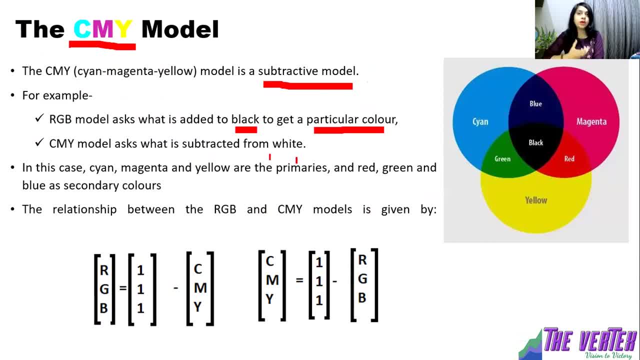 it will ask what should be subtracted from white to get particular color. In this case, cyan, magenta and yellow are primary color and red, green and blue are secondary colors. So in RGB model, red, green and blue are primary and cyan, magenta and yellow are secondary colors. 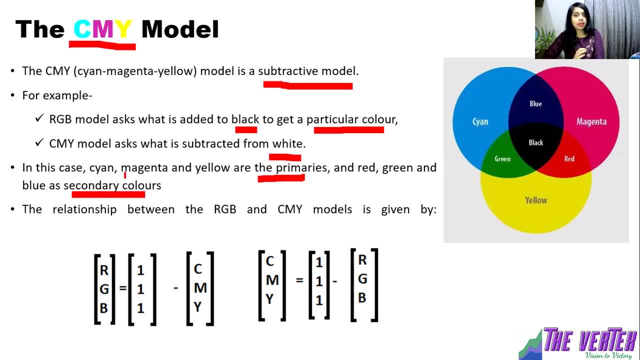 And in CMY model, CM and Y are primary colors and red, green and blue are secondary colors. So, as I have shown you earlier also, when we add magenta and cyan, we get blue. When we add magenta and yellow, we get red. 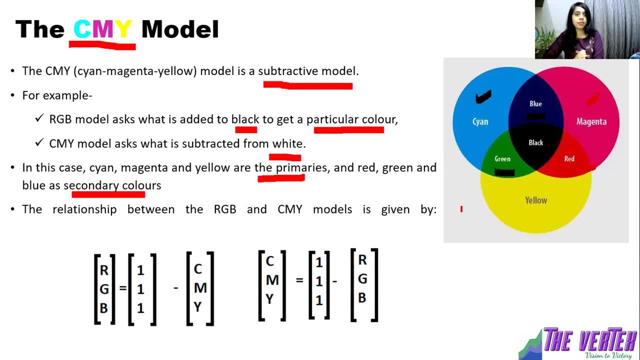 And when we add cyan and yellow we get green. Now how to convert one RGB model into CMY model or CMY model into RGB model. That means how to convert one color model into another color model. So formulas are given If you want to convert CMY into RGB. 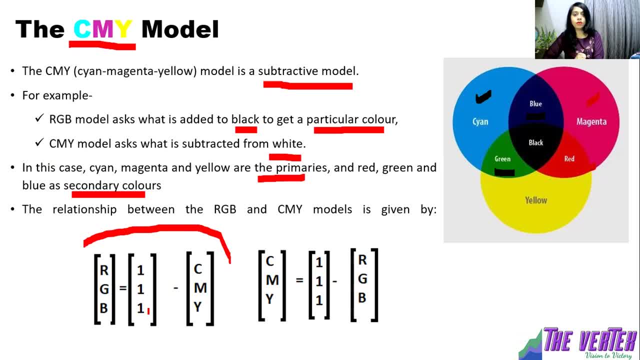 you have to subtract each value of CMY from 1.. And if you want to convert RGB into CMY, you have to subtract RGB from 1.. Now the question is how to convert these values from 1.. As I said, RGB values varies from 0 to 255. 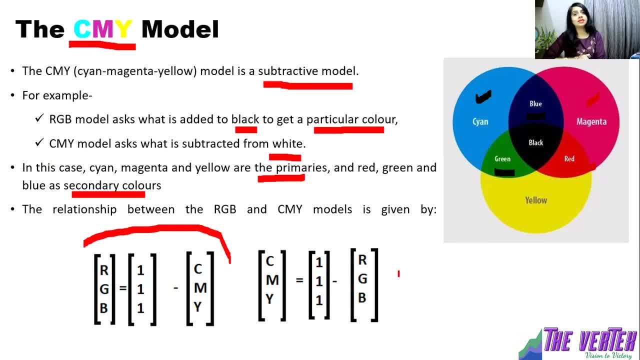 So for doing this, we have to normalize these colors. How do we normalize? We subtract the RGB value by 255.. We normalize it and then we subtract it from 1.. So I will show you one of the examples. So what is the example? 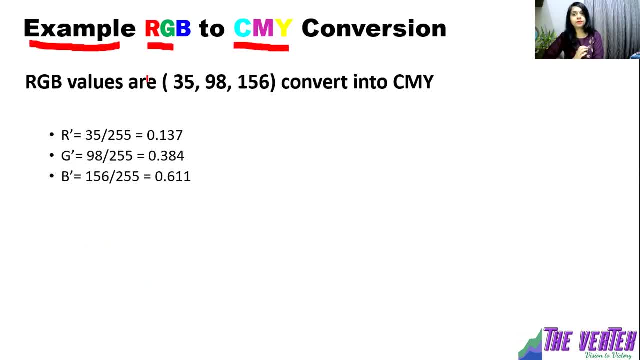 How to convert RGB into CMY. So, for example, it is given RGB values of 35,, 98 and 156.. What is meaning? This is red, this is green and this is blue value And we have to convert it into CMY. 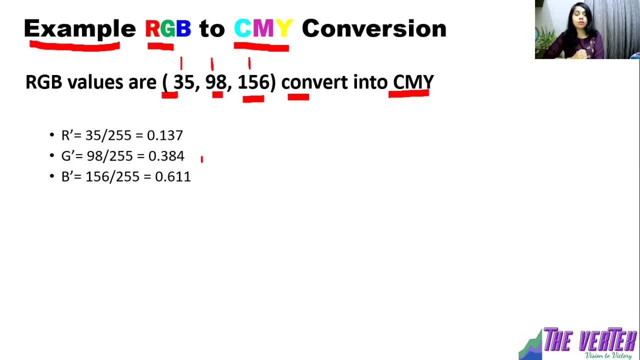 So first, before starting, we have to normalize this. How to normalize this? So I will calculate R', that is 35 divided by 255.. We will get this. Then G', that is 98 divided by 95 divided by 255. 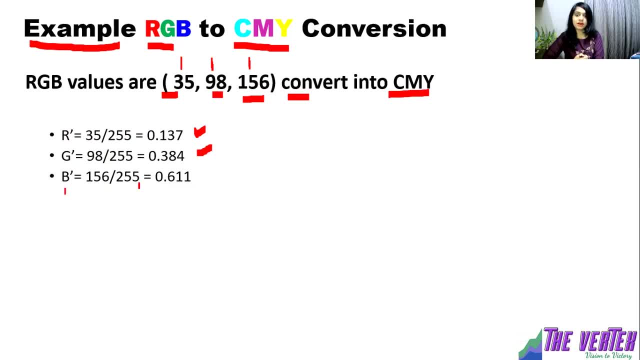 We will get this And blue. that is 156 divided by 255.. We will get 611.. After normalization, then we have to use the same formula that I have shown earlier. If you want cyan, then 1 minus R, that is 0.137.. 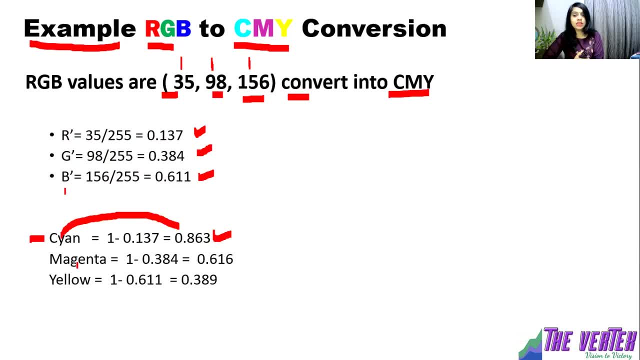 So you will get value of cyan, Then magenta color value, So 1 minus green, that is 1 minus 0.384.. So you will get this And yellow, forgetting yellow, you have to subtract 0.611 from 1.. 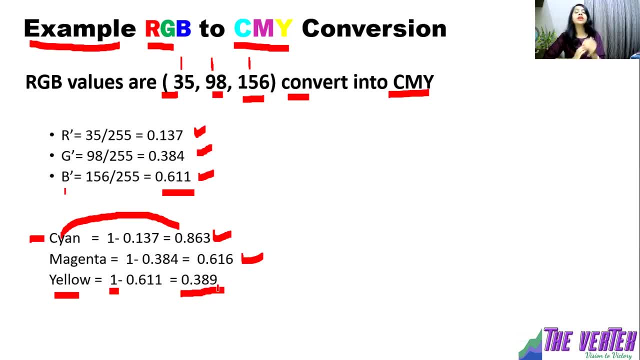 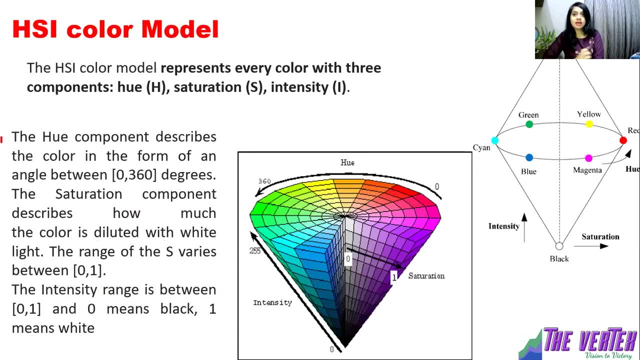 So you will get 0.389.. So this is how you can convert RGB to CMY. Now next color model is HSI color model. What is HSI color model? HSI color model represents every color with three components, That is, hue, saturation and intensity. 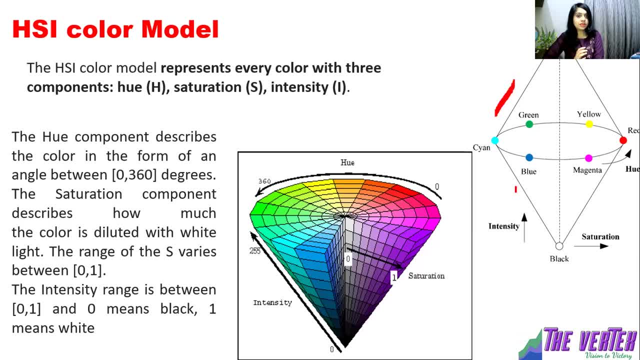 Now here this coordinate system for HSI model is shown. You can see here the saturation is varying in this direction. This end represents black, This upper end represents white. Intensity is increasing in this direction. That means here the intensity is lowest. 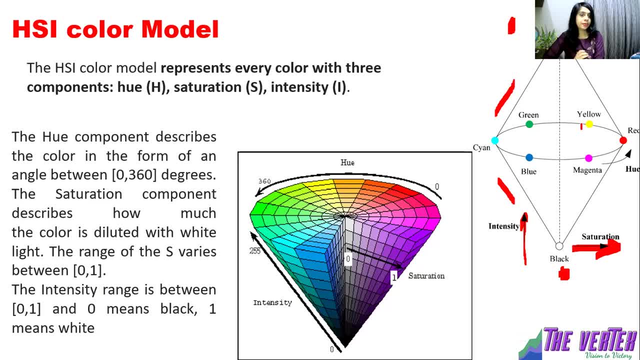 And at the top intensity is highest Colors you can see at this end there is red color, then yellow, green, cyan, blue and magenta. So there are rings of colors. If you want to have a detailed look, you can see here. this cone is represented here. 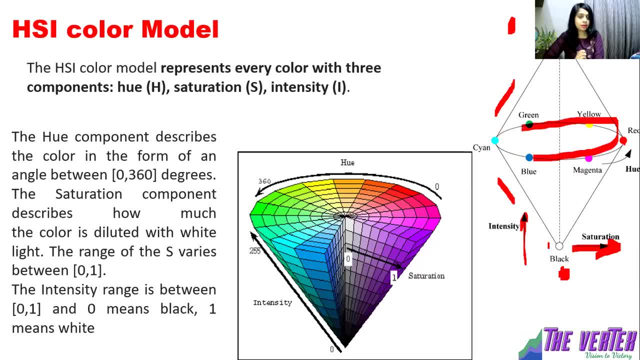 This cone. whatever is shown here, This particular cone is represented in this diagram. You can see the saturation is increasing in this direction. The saturation varies from 0 to 1.. As I have told earlier, also, highest value of saturation gives you the original color. 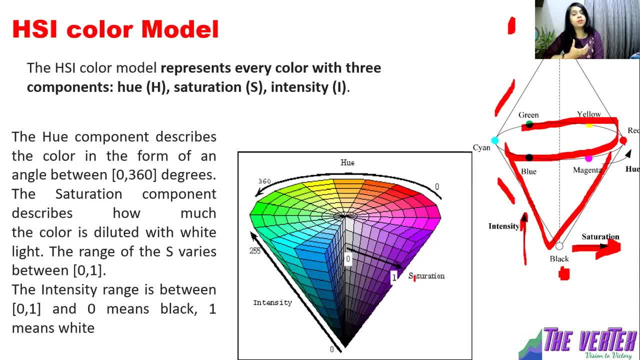 or original level or original color of that particular color. That means if saturation increases you will get the original form of that color And when saturation decreases you will get a pale form or dull form of that particular color. The U component describes the color in the form of angle between 0 to 360 degree. 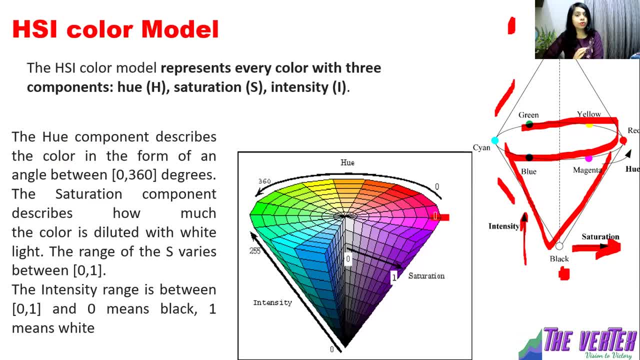 So if you see U as I told you, U represents the outer ring. Outer ring means again it is the purest form of that particular color family. So again U will change as an angle. So angle here U is 0 degree and in this direction. 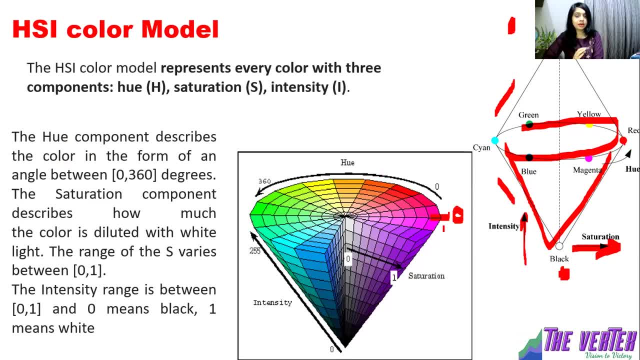 it will rotate like this and here again it will comes to 360 degree. So U the U component describes the color in the form of angle that varies from 0 to 360.. The saturation component describes how much color is diluted with white light. 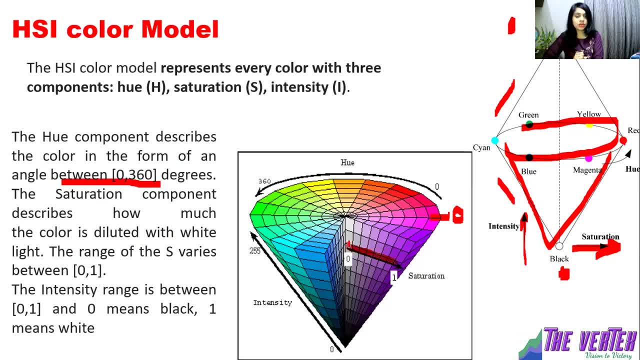 As I have shown you, in this direction the saturation is diluted, In this direction. here it is in the purest form. So saturation, here it is, the color is in its purest form. The range of saturation varies between 0 to 1.. 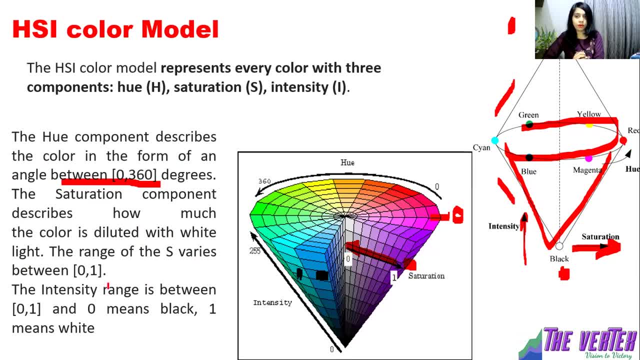 0 means it is in pure form, 1 means it is pure form, The intensity, intensity you can see, I have shown you intensity varying in this direction. That means on the downside it is black, It is the intensity is minimum, and on the upper side, 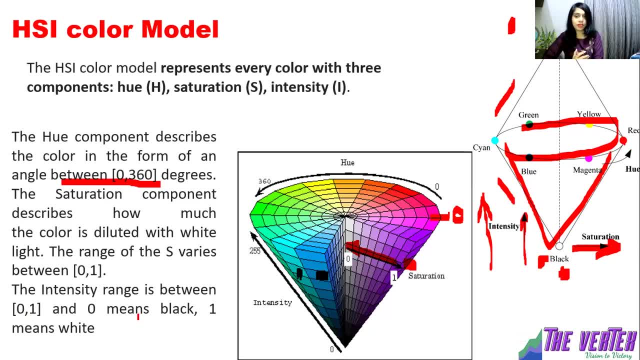 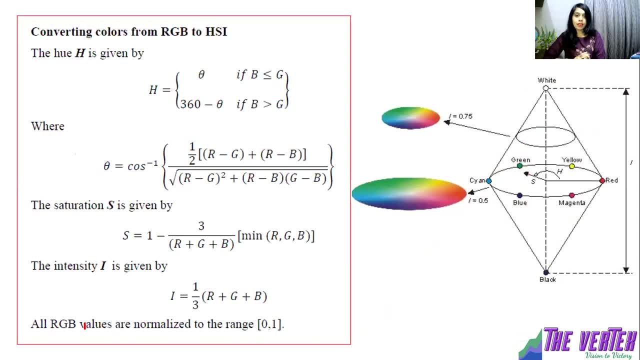 it is highest. The intensity ranges again between 0 and 1.. 0 means black and 1 means white. So this represents HSI color model. Now what are the formula for converting colors from RGB to HSI? Suppose I have RGB colors and I want to convert it into HSI model. 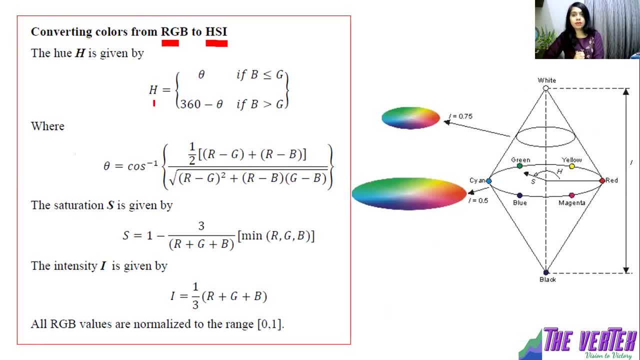 So there are formulas: The UH is given by H is equal to theta, If blue is less or equal to green. and if blue is greater than green, then you have to use this value: 360 minus theta, Where theta for theta. 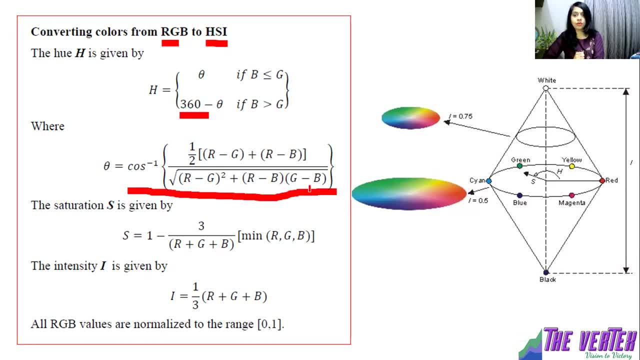 the formula is given. We have to use this formula. Then the saturation S. for saturation, Again the formula is given: S is equal to 1 minus 3 upon R plus G plus blue, and minimum of R, G, Y means whatever is the smallest that you have to multiply with this formula. 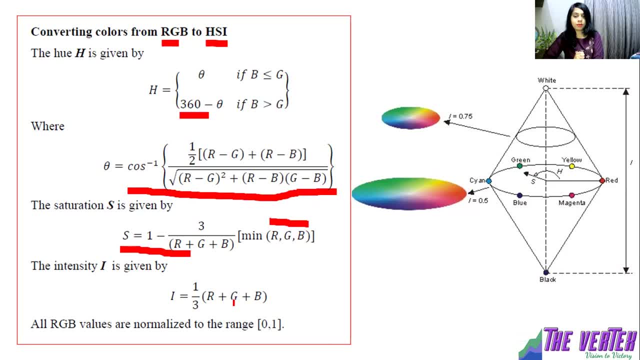 And intensity I is given by R plus G plus B, divided by 3.. Here again, you can see the HSI model with clarity here, as I have shown you. Here it is black, Here it is white, The U is this is the angle of U in this direction. 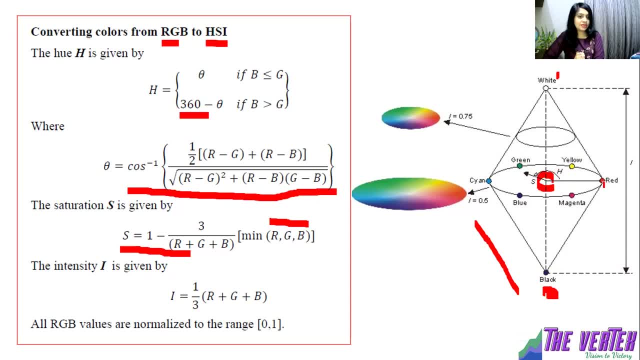 It is. it starts with 0. That means it starts with red and then ends with again red. The intensity you can see here intensity is supposed to be 0.5.. Here intensity is increased, That is 0.75.. 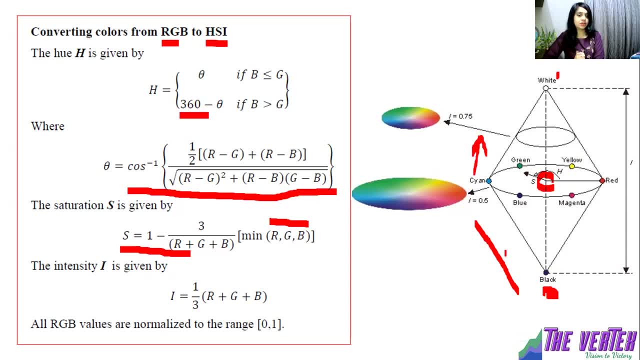 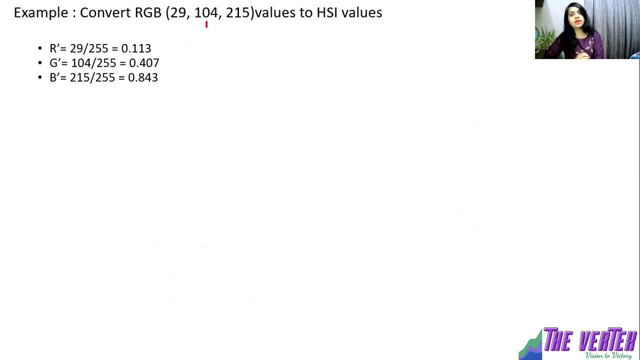 So intensity is increasing in this direction. Okay, Now let's solve an example: Convert RGB, So 29104 and 215 values to HSI. So before starting what we will do first, we will normalize these values by dividing by 255. 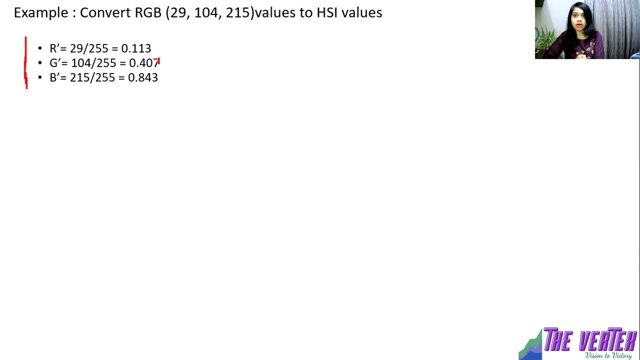 So we have divided by 255 and we have got these values of new values of R, G and B. Now the intensity I is given by I is equal to 1, by R plus G plus B is equal to G plus B. Very simple.